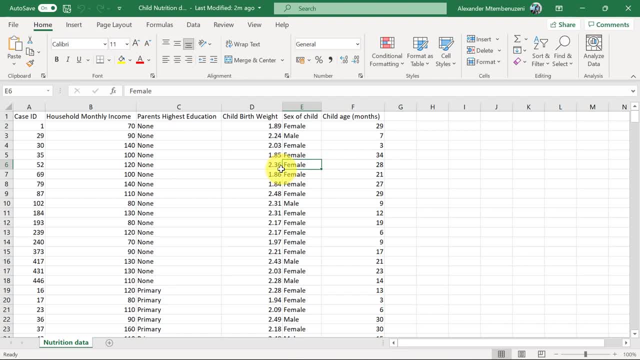 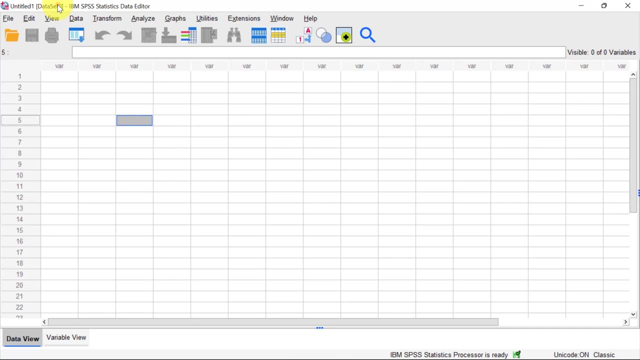 you can see, the data is in Microsoft Excel format, so we first of all need to import this into SPSS. I have provided a link to this dataset in the comments below, where you can download it for your practice. So the first thing is I'm gonna go ahead and close this Right. so now we're in SPSS. 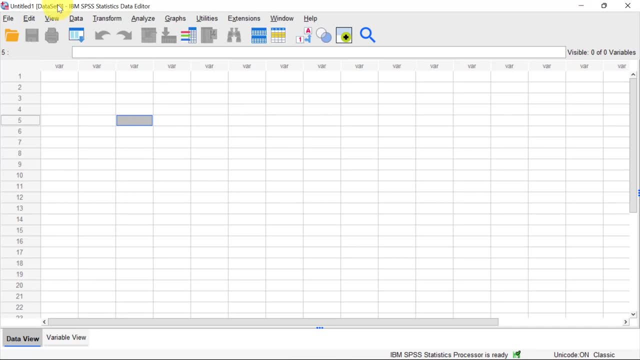 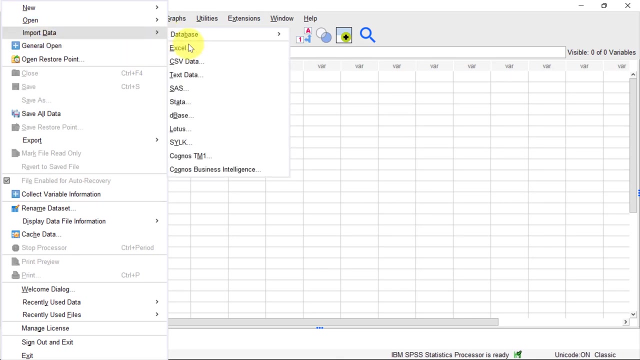 I have also provided a link to download the trial version of the latest version of SPSS For your practice. So now to import data that we have in Microsoft Excel into SPSS, the first thing you need to do is go to file and go to import data and select Excel. Now the next. 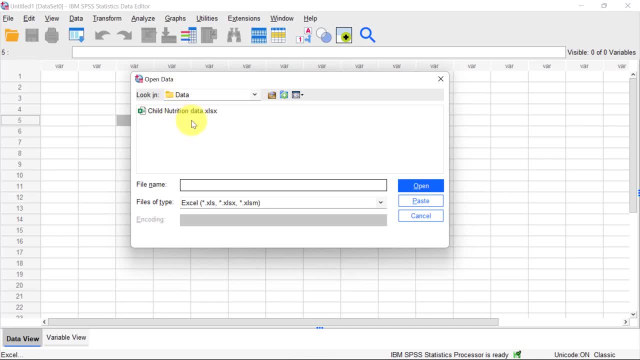 thing. you have this open data dialog box, so you have to go ahead and navigate to where you have your dataset. I already have my dataset right here- child nutrition data- so I just have to select it and click open. Now the next thing that's going to appear is the dialog box for reading. 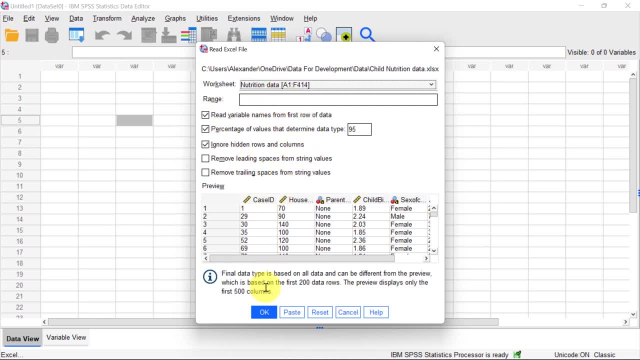 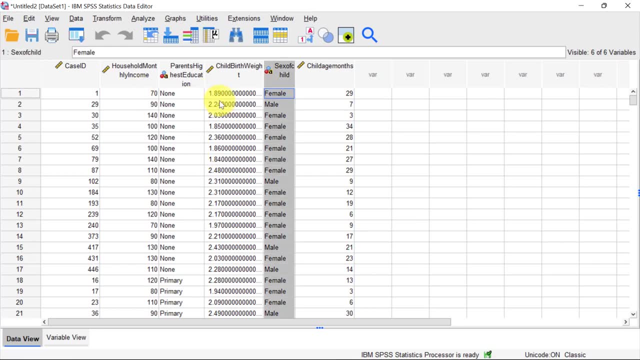 the Excel file. Everything here is perfectly fine, so I can just go ahead and click OK. So now you can see that we have our data in SPSS. So the very first thing that you need to do once you have the data is to take a look at the structure of your data. Especially, you have 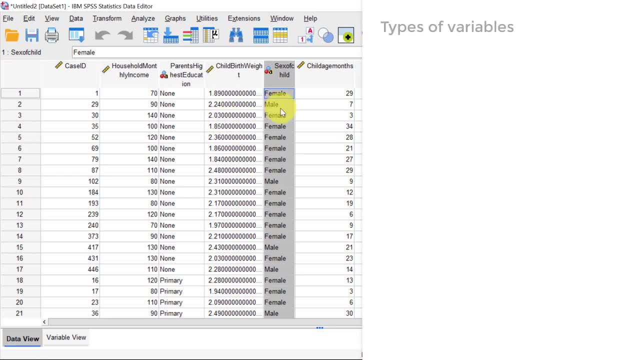 to look at the types of variables that you have. In general, there are two different types of variables. You have categorical variables, which are variables that are represented by words and have very few categories in most cases. An example is sex of child, which has only two values of female and male, and you have parents highest education. 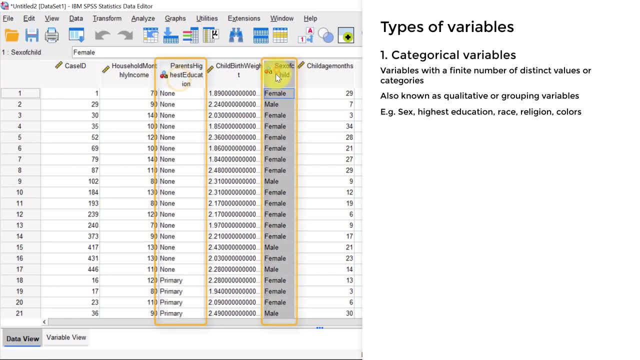 with quite a number of categories. So these are categorical variables. On the other hand, you have continuous variables, also known as quantitative variables. These variables measure quantities. For example, household monthly income is in US dollars and child birth weight is measuring the weight in kilograms and child age in months is measuring time in the number of months. Now the way 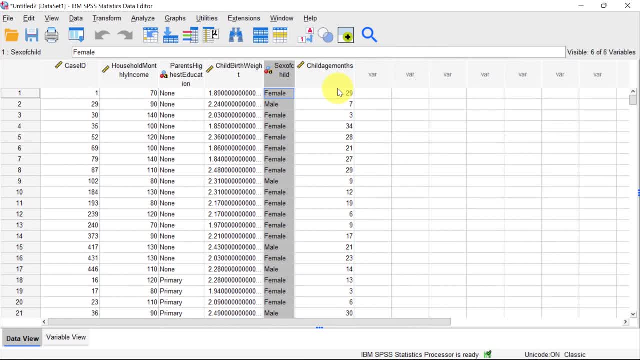 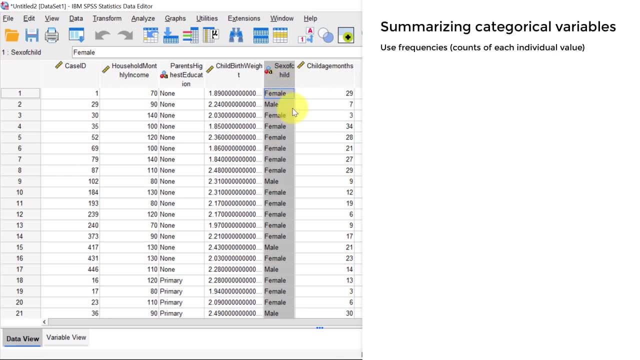 categorical variables is in most cases, different from the way that we summarize continuous variables. Let's start with categorical variables. The best way to summarize categorical variables is to use what are known as frequencies. These are simply counts of each category that you have in the categorical variable. As an example, sex of child here has two categories. We are interested. 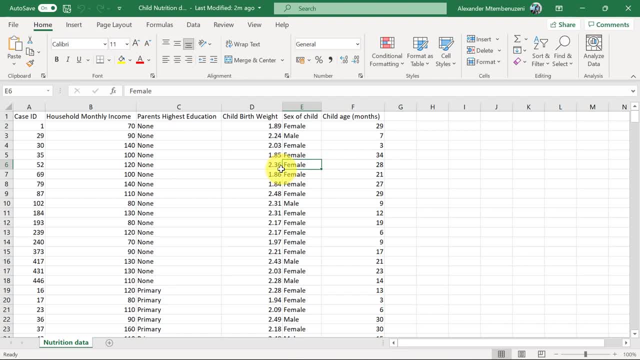 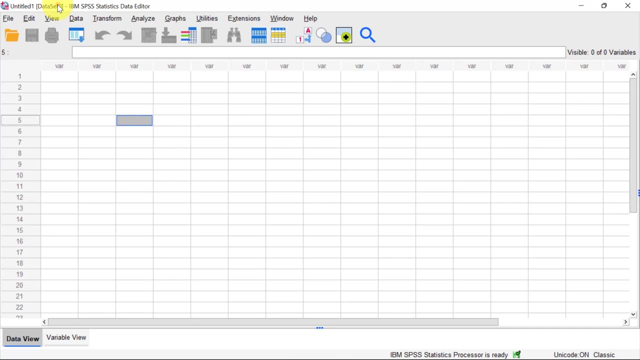 you can see, the data is in Microsoft Excel format, so we first of all need to import this into SPSS. I have provided a link to this dataset in the comments below, where you can download it for your practice. So the first thing is I'm gonna go ahead and close this Right. so now we're in SPSS. 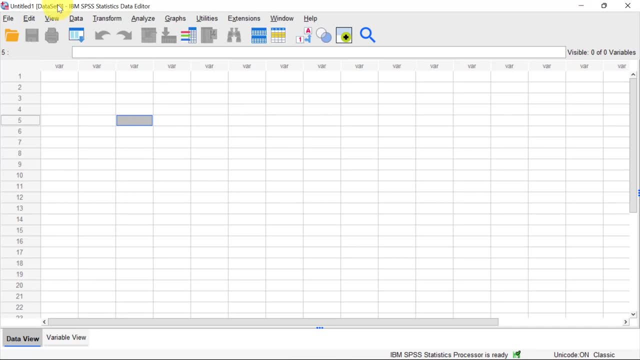 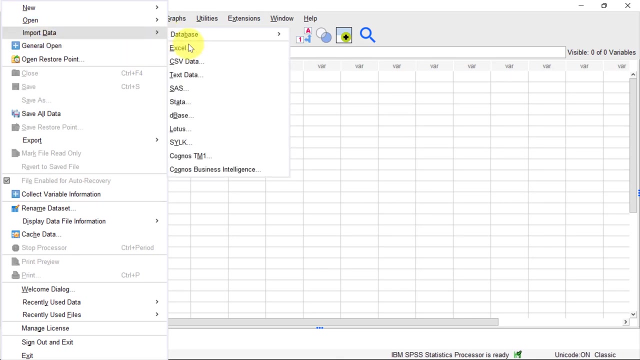 I have also provided a link to download the trial version of the latest version of SPSS For your practice. So now to import data that we have in Microsoft Excel into SPSS, the first thing you need to do is go to file and go to import data and select Excel. Now the next. 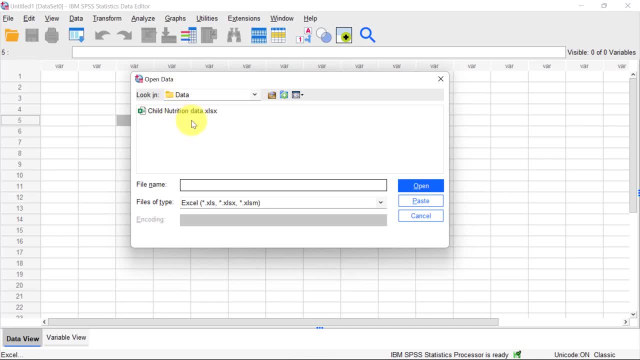 thing. you have this open data dialog box, so you have to go ahead and navigate to where you have your dataset. I already have my dataset right here- child nutrition data- so I just have to select it and click open. Now the next thing that's going to appear is the dialog box for reading. 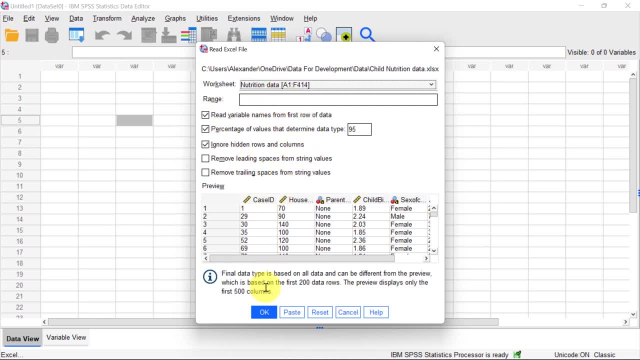 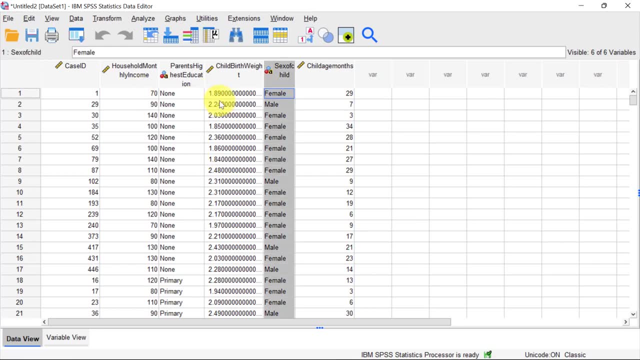 the Excel file. Everything here is perfectly fine, so I can just go ahead and click OK. So now you can see that we have our data in SPSS. So the very first thing that you need to do once you have the data is to take a look at the structure of your data. Especially, you have 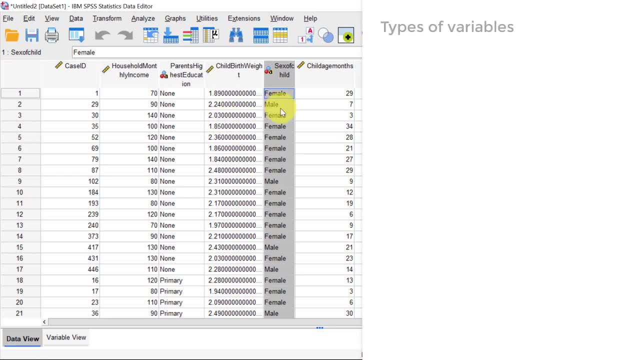 to look at the types of variables that you have. In general, there are two different types of variables. You have categorical variables, which are variables that are represented by words and have very few categories in most cases. An example is sex of child, which has only two values of female and male, and you have parents highest education. 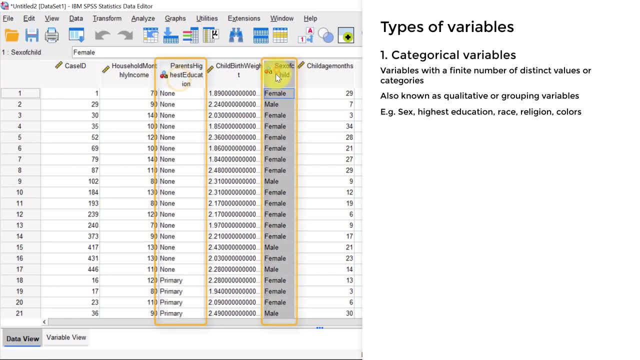 with quite a number of categories. So these are categorical variables. On the other hand, you have continuous variables, also known as quantitative variables. These variables measure quantities. For example, household monthly income is in US dollars and child birth weight is measuring the weight in kilograms and child age in months is measuring time in the number of months. Now the way 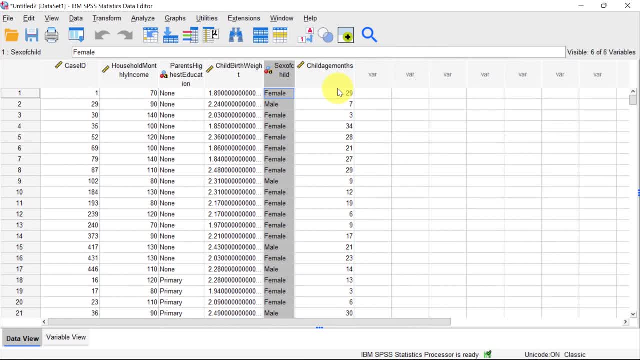 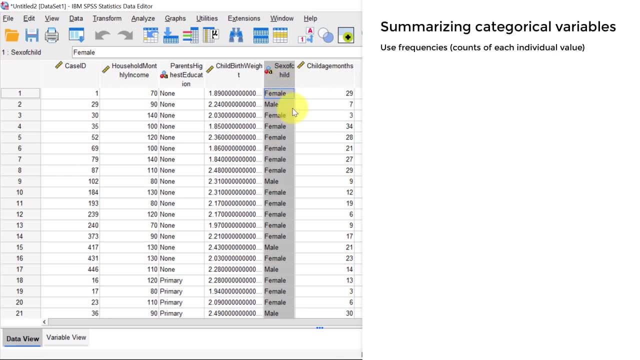 categorical variables is in most cases, different from the way that we summarize continuous variables. Let's start with categorical variables. The best way to summarize categorical variables is to use what are known as frequencies. These are simply counts of each category that you have in the categorical variable. As an example, sex of child here has two categories. We are interested. 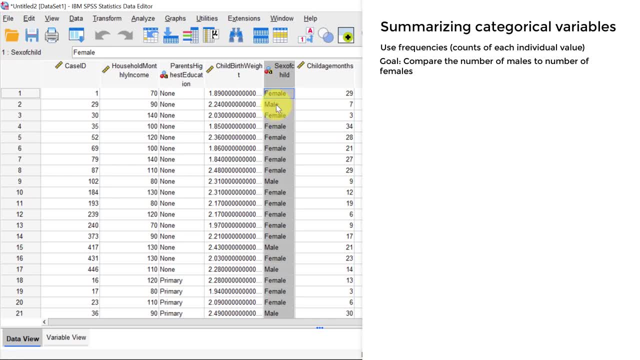 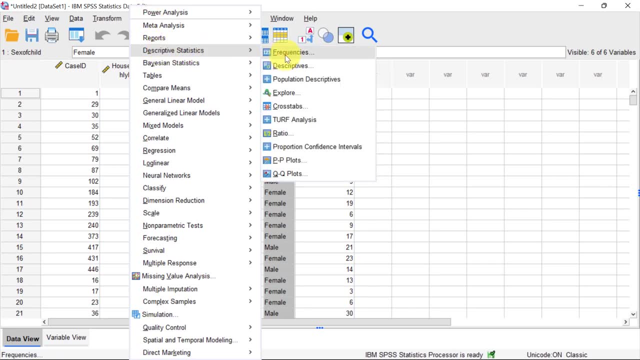 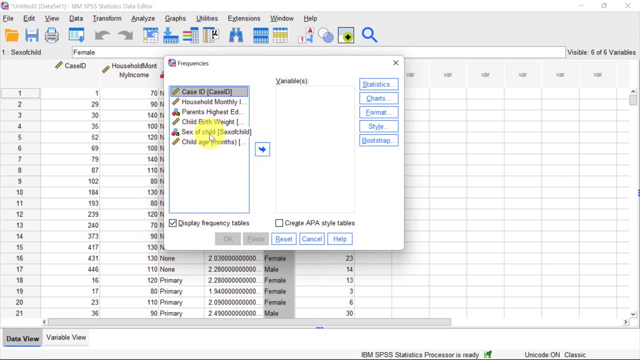 to find out how many females there were and how many males there were. To do that, you just go ahead and click analyze on the menu, Go to descriptive statistics and click frequency. On the left hand side you have a list of variables that we have in the data set. So it's as simple as 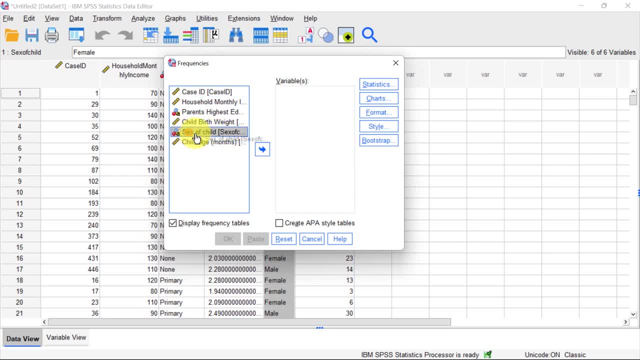 dragging the variable that you want, in this case sex of child, and drop it on the right hand side where it says variables. We can also drag and drop the variable parents- highest education and just put it in there as well. Now, the next thing you might want to do is to go to charts and then turn on. 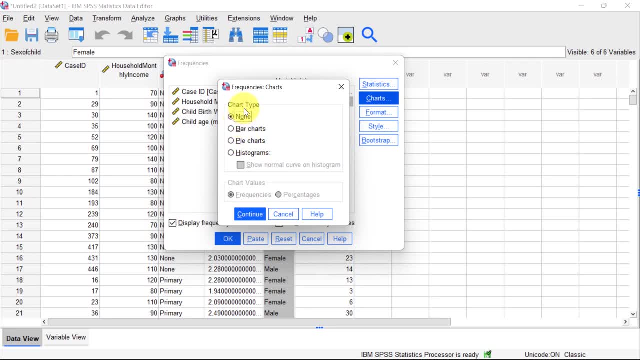 either a bar chart or a pie chart, which are appropriate for the variable that we are using so far. that is a categorical variable, So I'll just pick a bar chart and click continue. Trust me, this is all you need to do here and you can go ahead and click. okay. 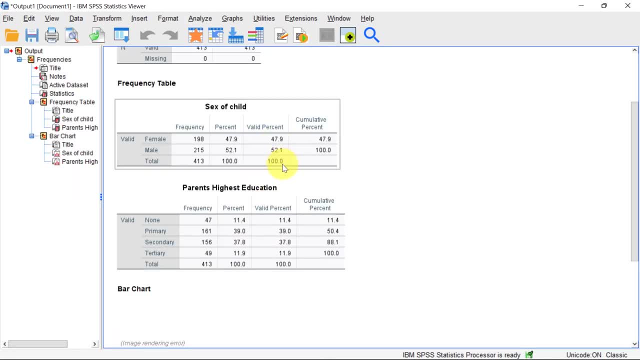 Now, in just those few clicks, you can see that we have our analysis right here. So to interpret this: we had 198 female children and 215 male children, and here those numbers are being presented in percentages. So 47.9 percent are female and 52.1 percent are male. If this variable had a few 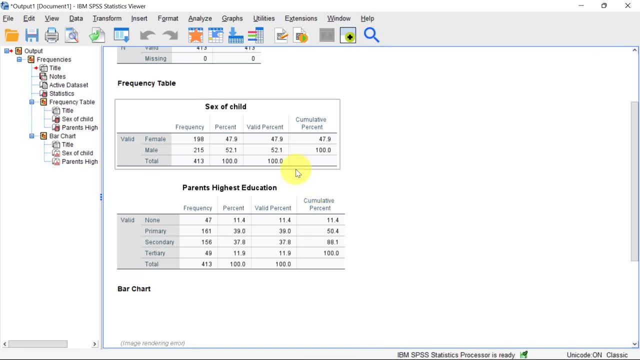 people who did not respond to the question. the best percent to use is this one here called valid percent, which is expressed out of only those people who responded in that question. Now the question is: how do we present this in our report? So I'm going to go. 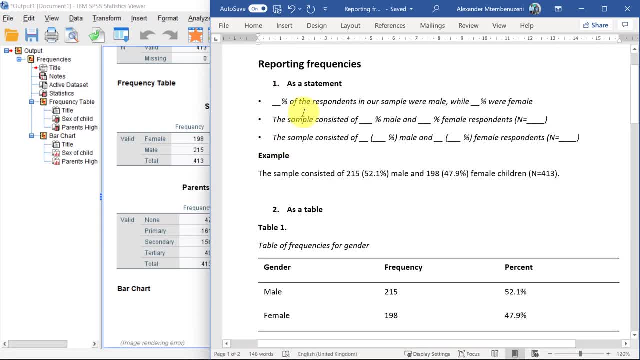 ahead in Microsoft word. So at the top we have several templates of how you can write that. but as an example I could say the sample consisted of 215 and in brackets we have the percentage and 198 and we have the percentage in brackets- female children. And here the error is. 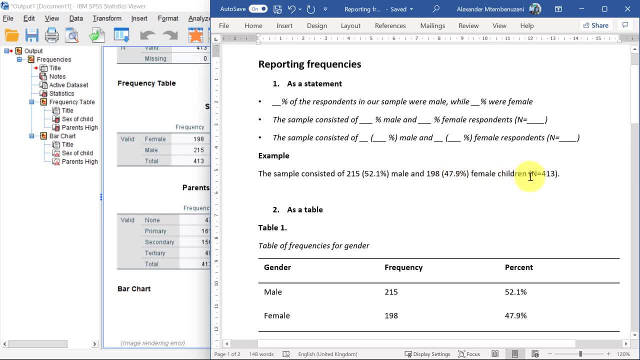 99, М and 998, and we have the percentage in brackets, female children, and here the I am providing the total N, that is the total number of children that we have in the data set, which is 413.. With that, that's perfect. 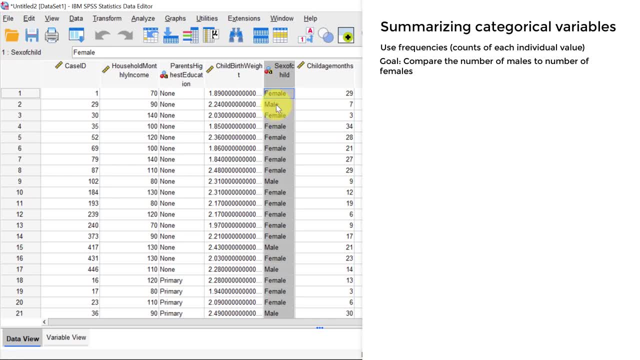 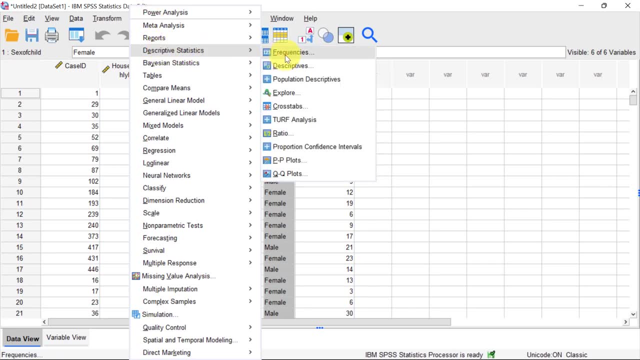 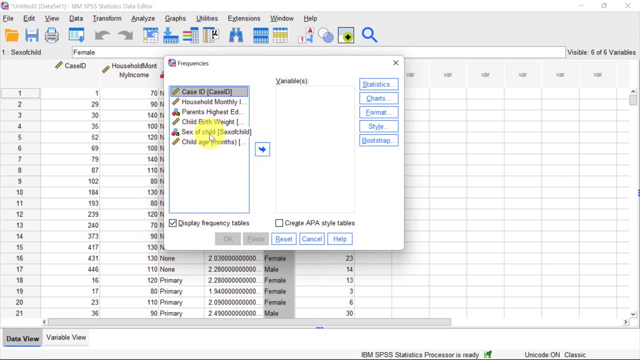 to find out how many females there were and how many males there were. To do that, you just go ahead and click analyze on the menu, Go to descriptive statistics and click frequency. On the left hand side you have a list of variables that we have in the data set. So it's as simple as 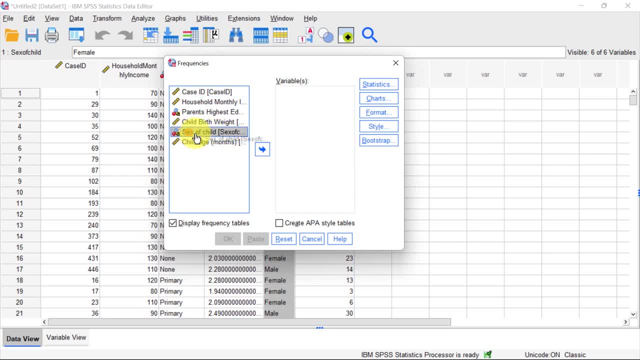 dragging the variable that you want, in this case sex of child, and drop it on the right hand side where it says variables. We can also drag and drop the variable parents- highest education and just put it in there as well. Now, the next thing you might want to do is to go to charts and then turn on. 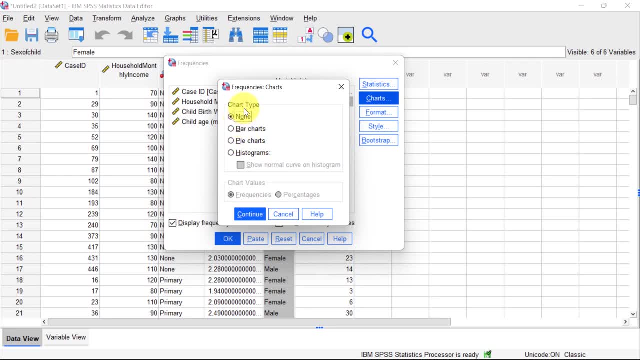 either a bar chart or a pie chart, which are appropriate for the variable that we are using so far. that is a categorical variable, So I'll just pick a bar chart and click continue. Trust me, this is all you need to do here and you can go ahead and click. okay. 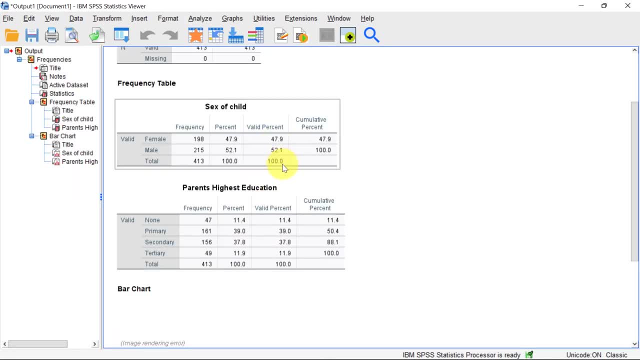 Now, in just those few clicks, you can see that we have our analysis right here. So to interpret this: we had 198 female children and 215 male children, and here those numbers are being presented in percentages. So 47.9 percent are female and 52.1 percent are male. If this variable had a few 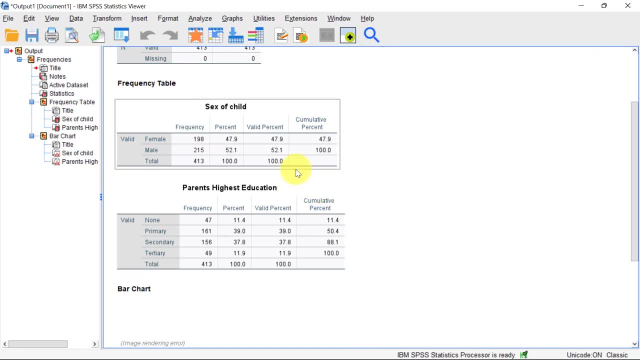 people who did not respond to the question. the best percent to use is this one here called valid percent, which is expressed out of only those people who responded in that question. Now the question is: how do we present this in our report? So I'm gonna go ahead. 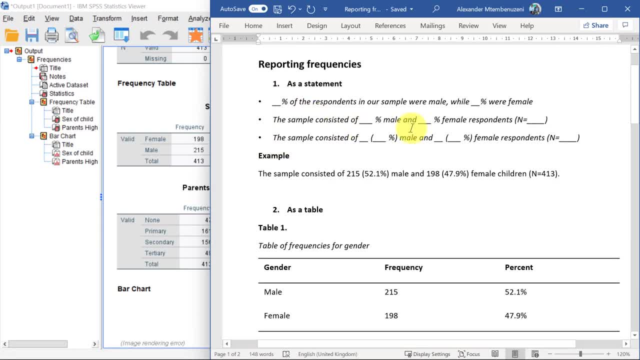 in Microsoft Word. So at the top we have several templates of how you can write that. but as an example I could say the sample consisted of 215 and in brackets we have the percentage male and 198 and we have the percentage in brackets female, children and here about 215 females and in brackets 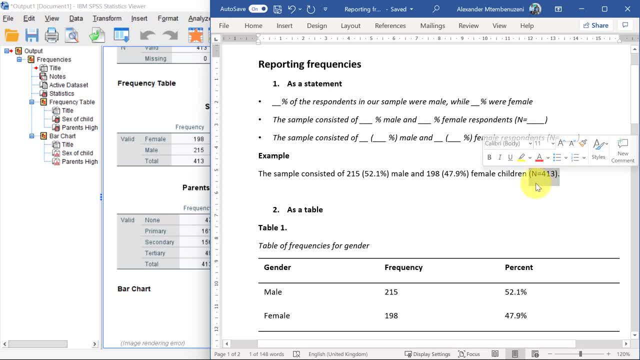 I am providing the total n, that is, the total number of children that we have in the data set, which is 413. with that, that's perfect. your dissertation or thesis or report is moving as a table. This is how you can present it, using the APA format now. 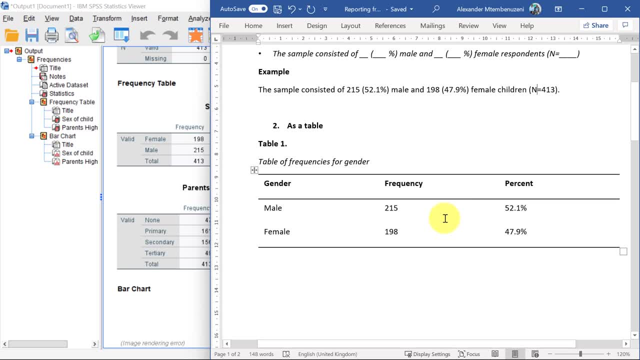 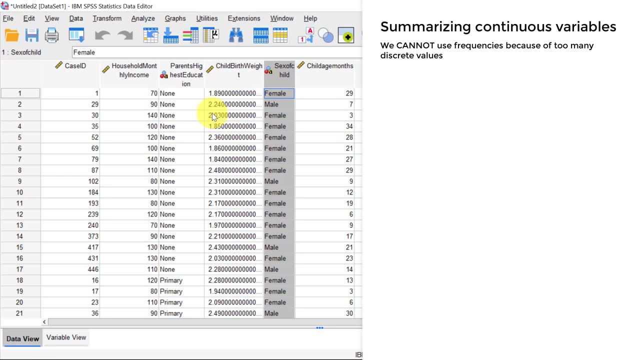 Let's go back and take a look at how we can summarize continuous variables. now, to summarize continuous variables, We cannot use frequencies, We cannot count each value, because in most cases for continuous variables You have so many different unique values in the variable. For example, if you take the variable child birth weight. 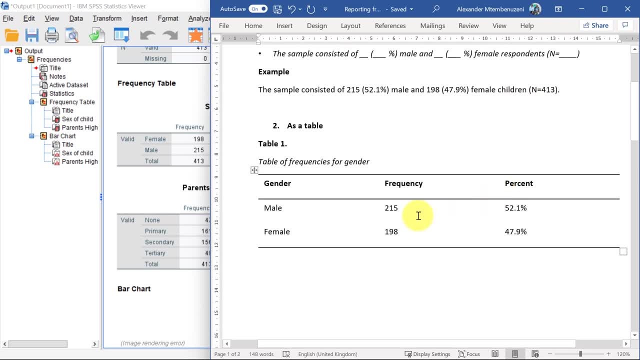 Your dissertation or thesis or report is moving As a table. this is how you can present it using the APA format. Now let's go back and take a look at how we can summarize continuous variables. Now, to summarize continuous variables, we cannot use frequencies. 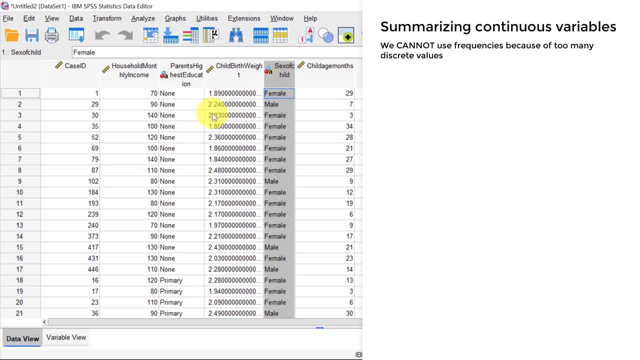 We cannot count each value because in most cases for continuous variables you have so many different unique values in the variable. For example, if you take the variable child birth weight, you have so many different birth weights for each individual child we have in the data set. 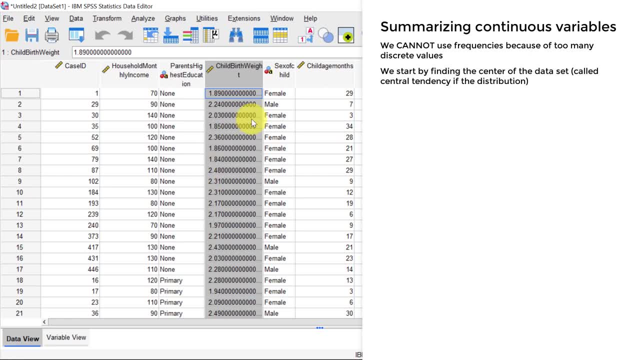 The best way in which you can summarize this is looking at the central point of the data set that we have in this variable. The idea behind that is that the number that is at the center of the data is the typical value in that data set. 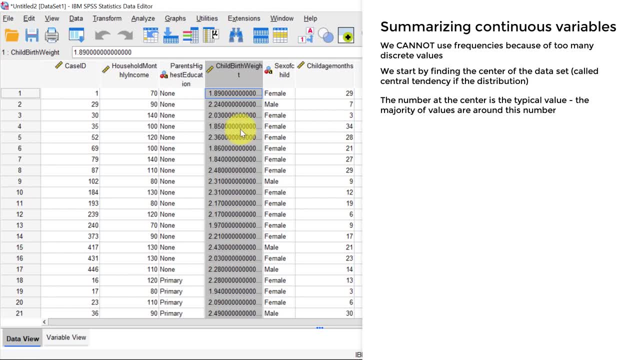 Or in other words, it represents the majority of the values that we have in the data set. The statistic that we can use for that is the mean. You know that simply as the average. So to summarize child birth weight using the mean, you have to click analyze on the menu, go to descriptive statistics and select frequencies. 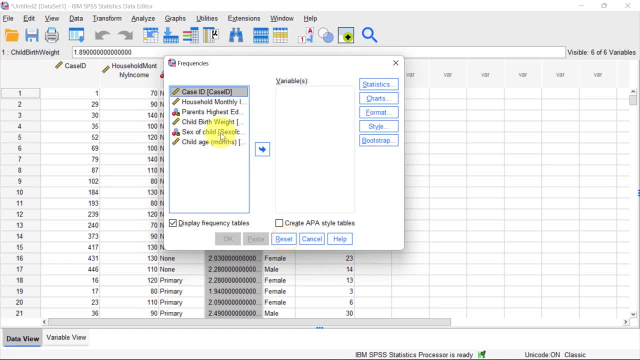 So the next thing I need to do here is click reset And then I'm going to drag and drop the variables I want to summarize, So in this case, child birth weight, But I'm also going to throw in household monthly income and child. 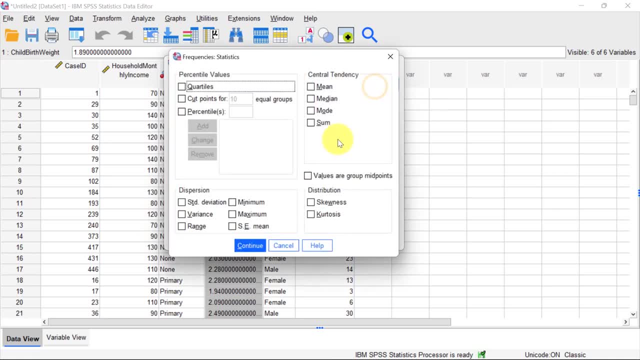 Age in months. Then the next thing is you go to statistics pattern and we're going to choose to produce the mean And of course in most cases you also want the standard deviation. Then I go ahead and click continue. The next thing: you can actually go into the charts and choose to produce a histogram. 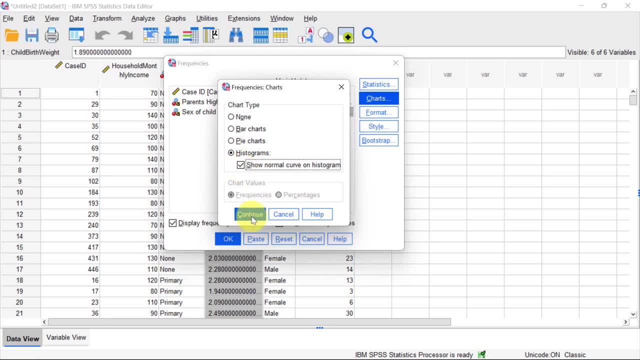 And of course, you might also want to show the normal curve on the histogram and click continue. Finally, you need to remove display frequency tables because, remember, we are dealing with continuous variables and then you click OK. So now, if you take a look at our output, 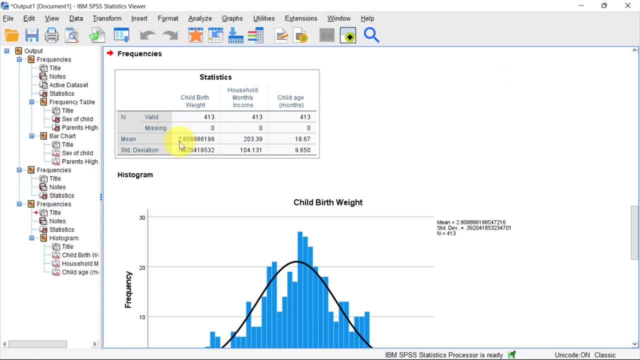 Right now. you can see that for child birth weight, the average is two point eight kilograms, but the standard deviation is zero point three nine. So how do we interpret that? A mean of two point eight means that the majority of the children weigh somewhere around two point eight kilograms. 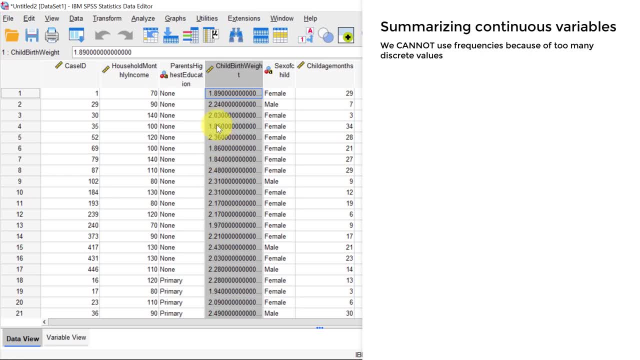 You have so many different birth weights for each individual child We have in the data set. the best way in which you can summarize this is looking at the central point of the data set That we have in this variable. The idea behind that is that the number that is at the center of the data is the typical value in that data set. 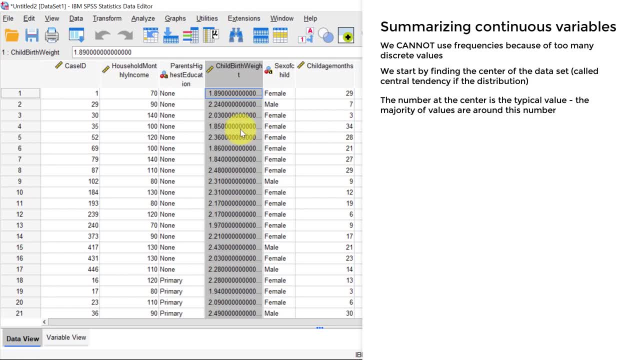 Or in other words, it represents the majority of the values that we have in the data set. The statistic that we can use for that is the mean. you know that's simply as the average. So to summarize child birth weight using the mean, you have to click analyze on the menu, go to descriptive statistics and select. 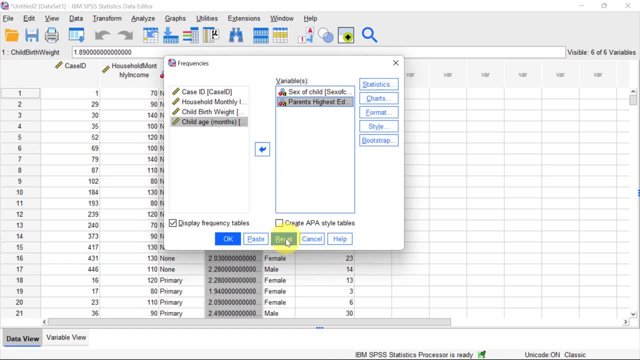 frequencies. So the next thing I need to do here is click reset and then I'm going to drag and drop the variables. I want to summarize, so in this case, child birth weight, But I'm also going to throw in household monthly income and child age in months. 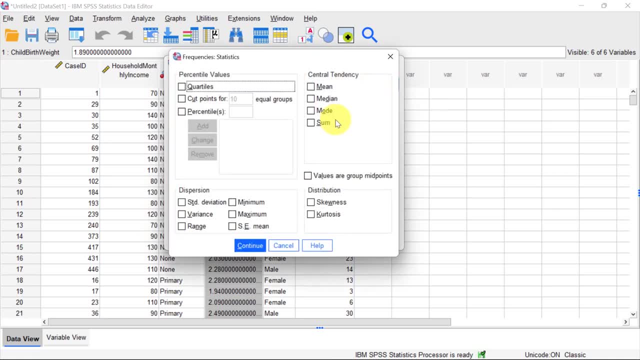 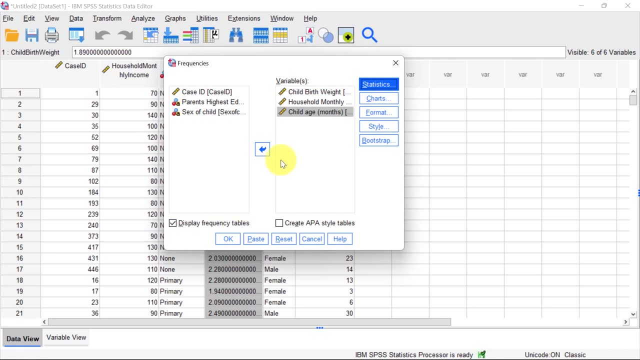 then the next thing is you go to statistics button and We're going to choose To produce the mean and of course in most cases you also want the standard deviation. Then I go ahead and click continue and the next thing, you can actually go into the charts and choose to produce a histogram. 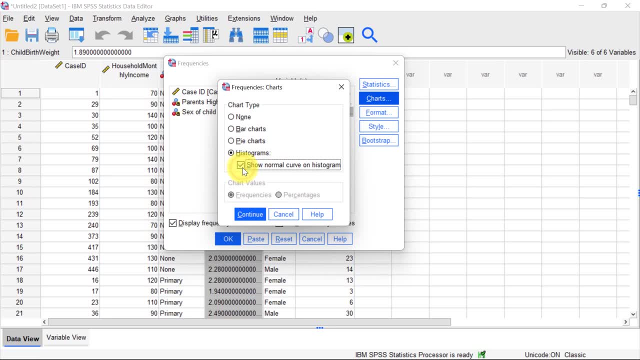 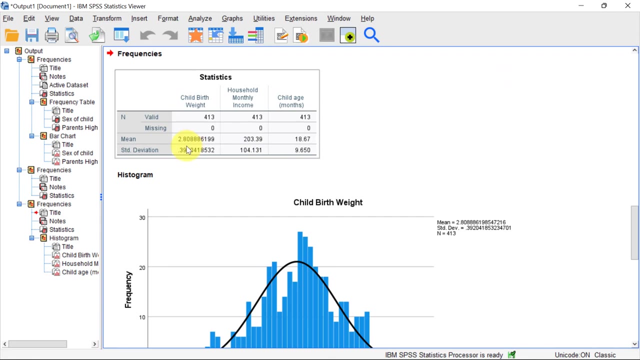 And of course, you might also want to show the normal curve on the histogram and click continue. Finally, you need to remove display frequency tables because, remember, we are dealing with continuous variables and then you click OK. So now, if you take a look at our output right now, you can see that for child birth weight, 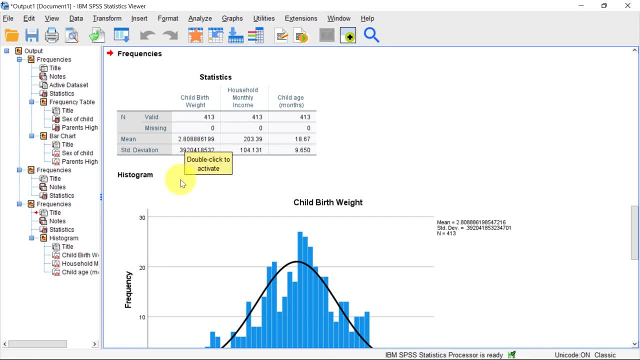 The average is 2.8 kilograms, But the standard deviation is 0.39. So how do we interpret that? a mean of 2.8 means that the majority of the children weighs somewhere around 2.8 kilograms. But just saying that is not enough. 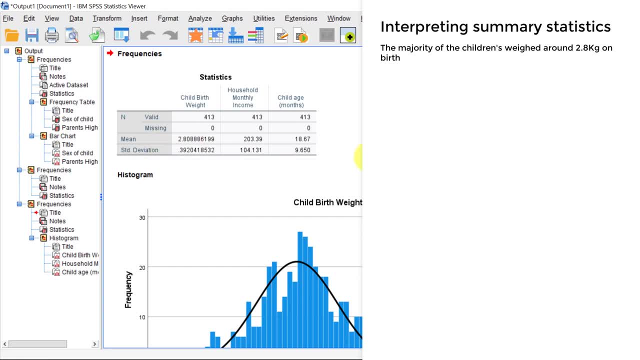 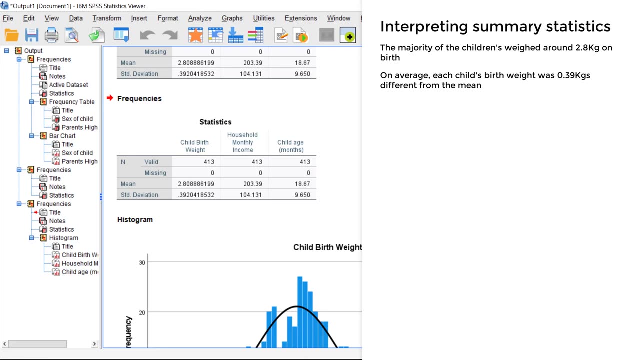 We also have to show how far apart the values are from each other, and that's why we need the standard deviation. So the standard deviation is telling us that, on average, the values are 0.39 kilograms away from the mean. So now the question is: how do we go ahead and actually report this in our thesis? 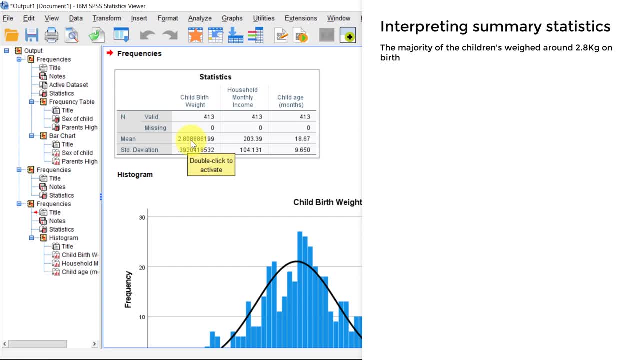 But just saying that is not enough. We also have to show how far apart the values are from each other, And that's why we need the standard deviation. So the standard deviation is telling us that, on average, the values are zero point three, nine kilograms away.